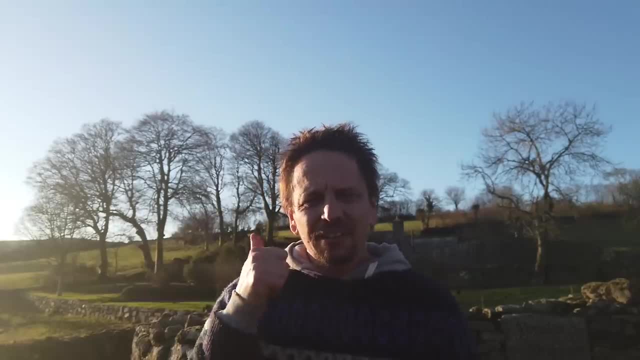 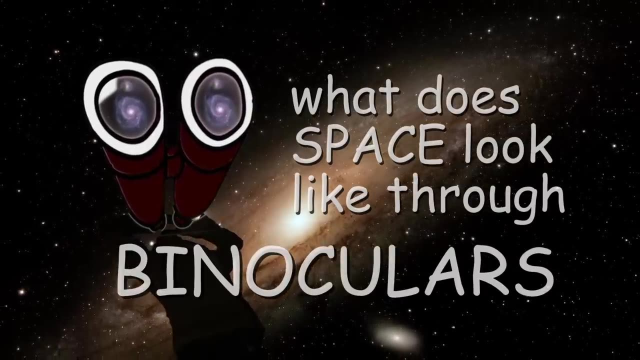 night sky. whether the two things are a success or a failure, We are going to know what it's like to look at space through binoculars. These, by the way, cost £69.00.. Wow, Wow, £69.00.. 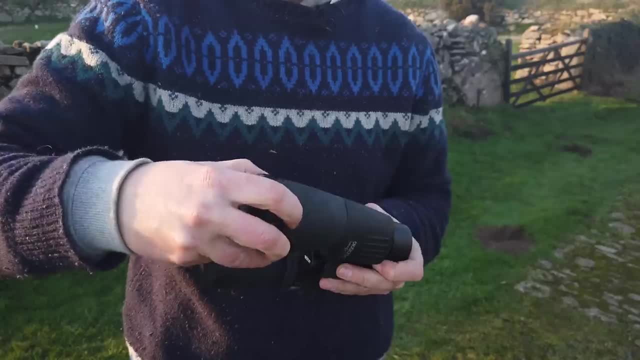 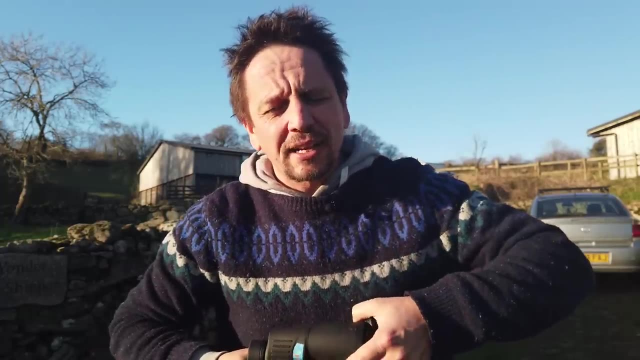 Apparently they're really good. One of the things that makes them good is they've got nice big 50mm lenses that let the light in and they're not mega zoomed in, They're only times seven magnification And that's pretty good for looking at the night sky, because 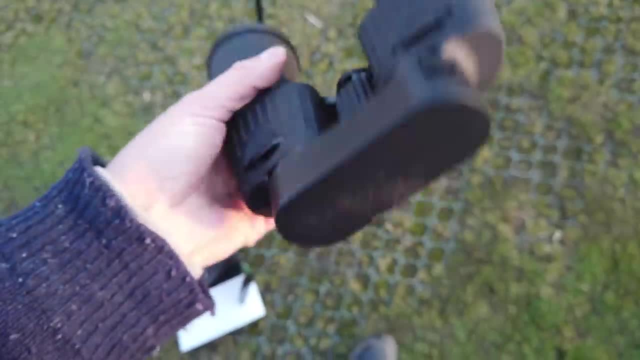 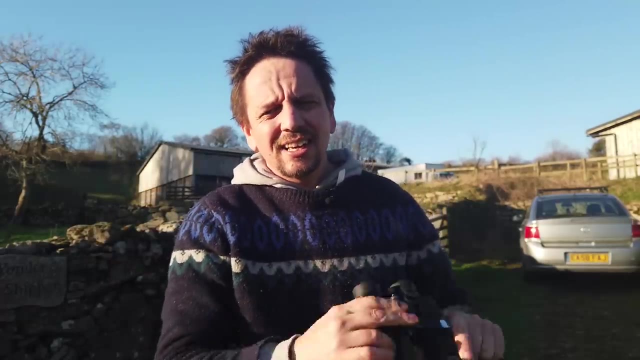 the more zoomed in you are, the less bright what you're looking at is So. it's like they're like big light buckets. Also, I believe, because they're not so zoomed in, you can handhold them without the wobble. 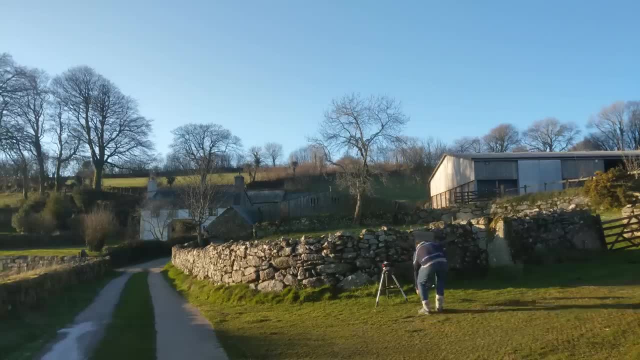 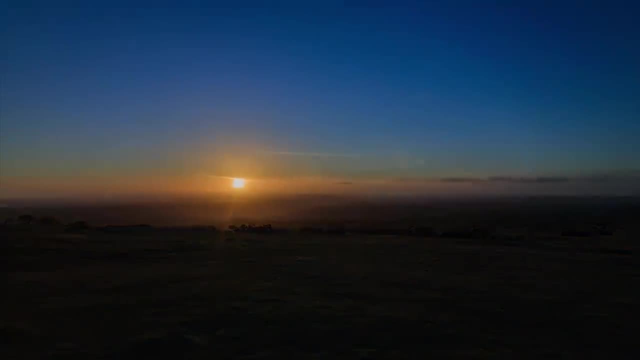 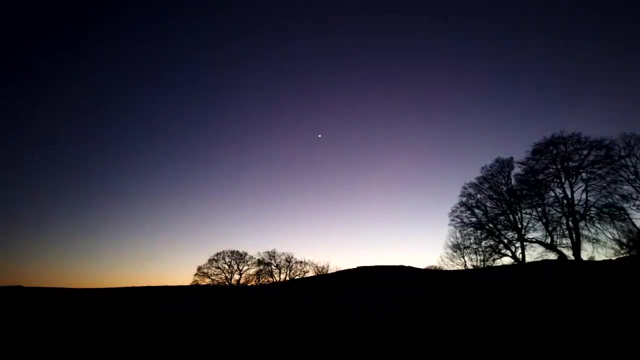 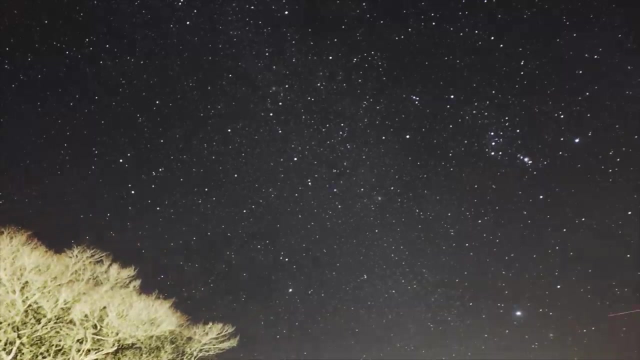 being too bad. So anyway, we're going to find out. All right, bring on the night. There's Venus, And coming out from behind those trees which are being lit up by the security light from a cow shed is the Milky Way. 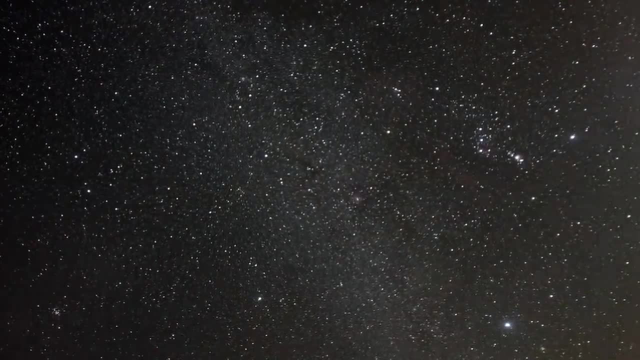 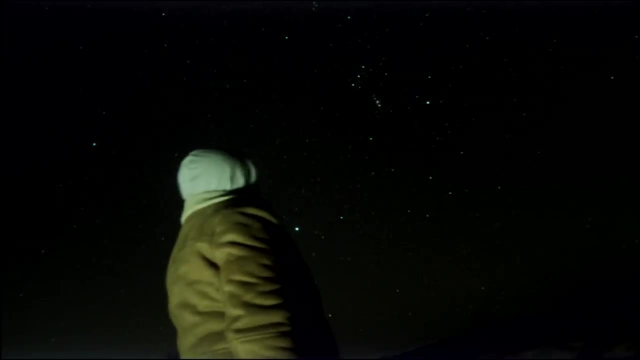 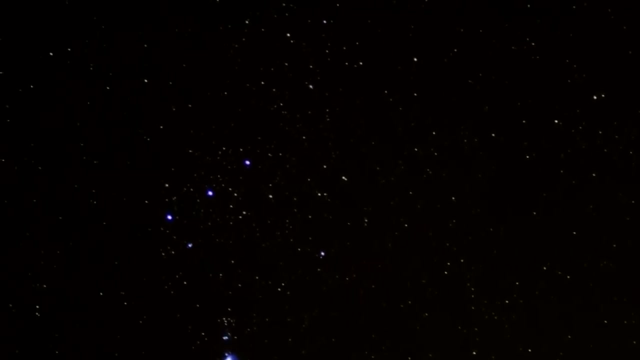 Look at that, And just in front of the Milky Way is my favourite constellation, Orion, is looking. I mean, he really is standing there, isn't he? He's a bloke standing in the heavens. Every astrophotographer loves Orion because there's so much cool stuff to photograph. 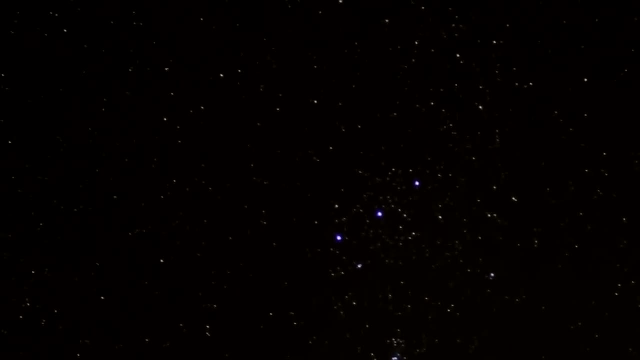 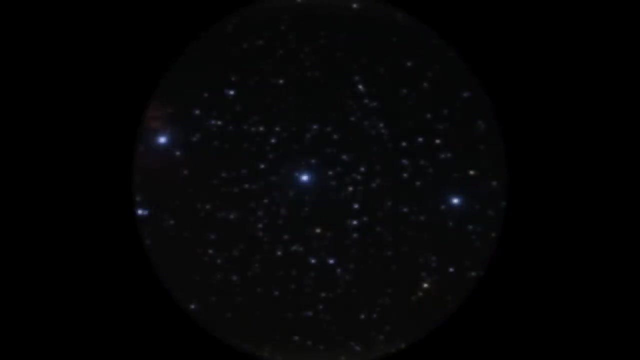 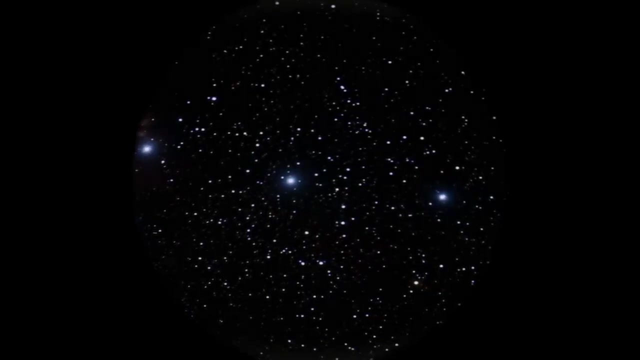 And I'm going to use those famous three stars of his belt to get focus. And it's our first opportunity to bring in BinoCam Absolutely swarming with stars. It's just so varied And, to be honest, it is far better than anything I'm getting with Astrocam or, in fact, any picture. 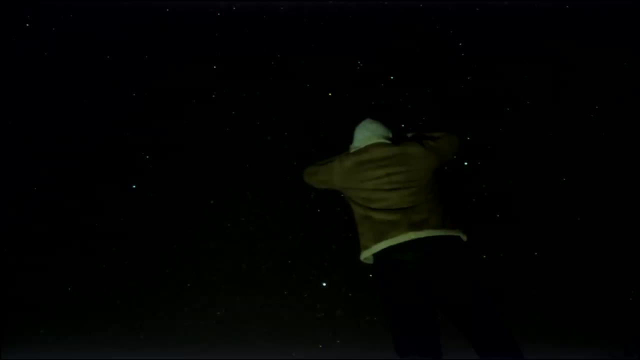 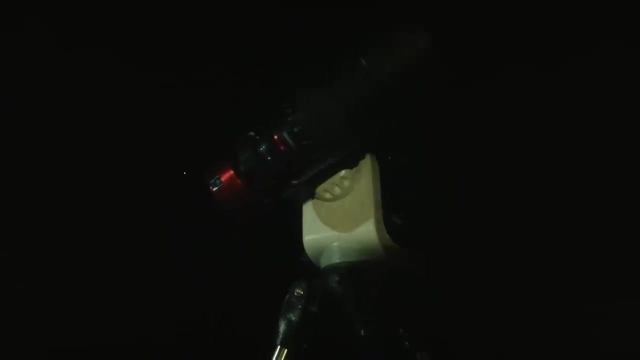 I've ever taken, And that's because the human eye has a thousand times better dynamic range than any camera. Just got to say it's fantastic. So BinoCam, brilliant at reproducing the binoculars field of view, but not so good atiem, At least. 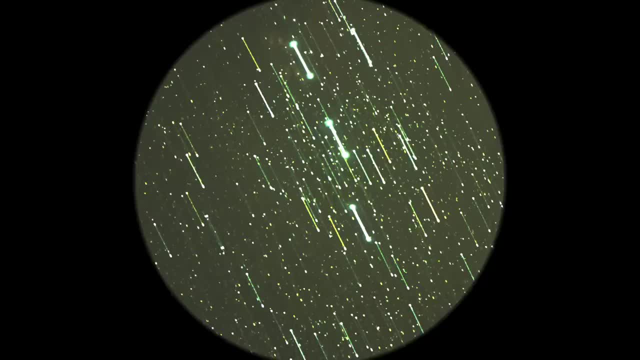 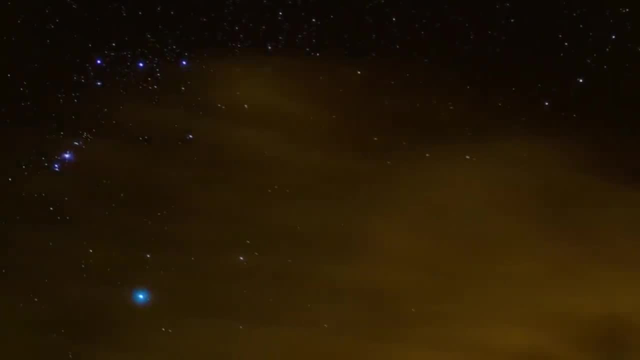 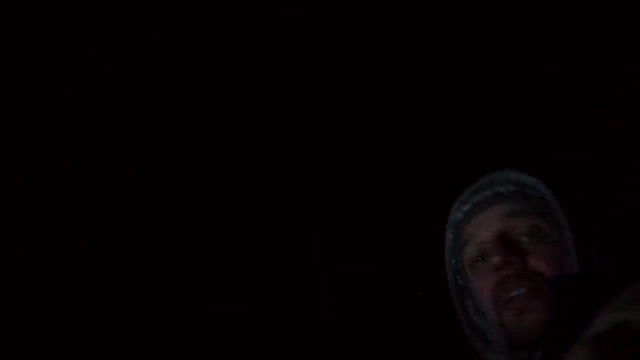 it's good, but not so good at reproducing the brightness of the stars. Ay, ay, ay. But cameras are supposedly far better at picking out the faint stuff. So just below the belt is the great nebula of Orion. That's the first place to go, I reckon. 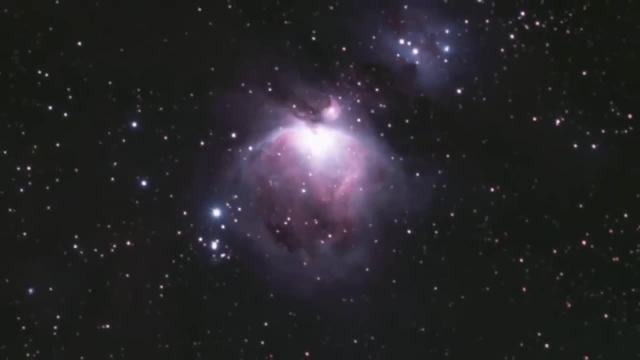 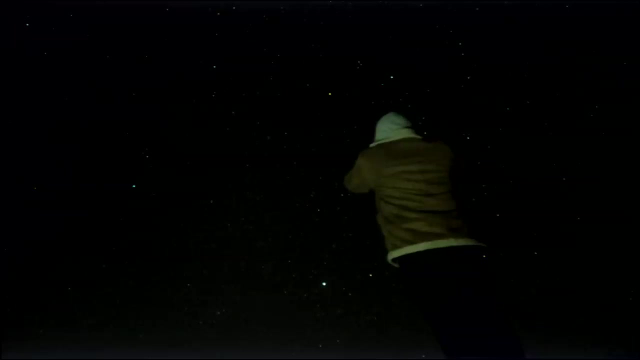 Here's what it looks like through a camera. This took over an hour to get, So the question is: how will our eyes and these binos do in? well, the blink of an eye, Oh yeah, yeah, there she is. 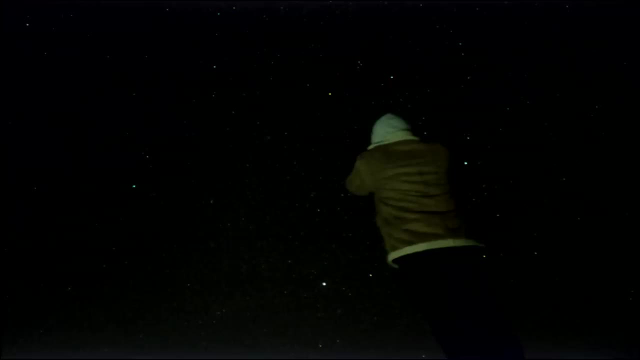 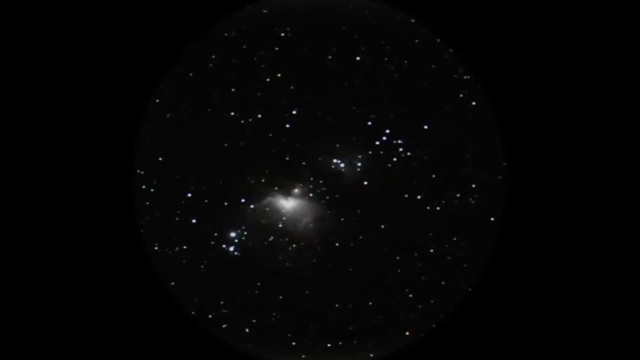 I can see it. It's a massive grey cloud. It looks like some kind of winged creature. Okay, this is my best attempt to grade binocam and show you what I saw. I admit it looks a little bit hokey, but there we go. 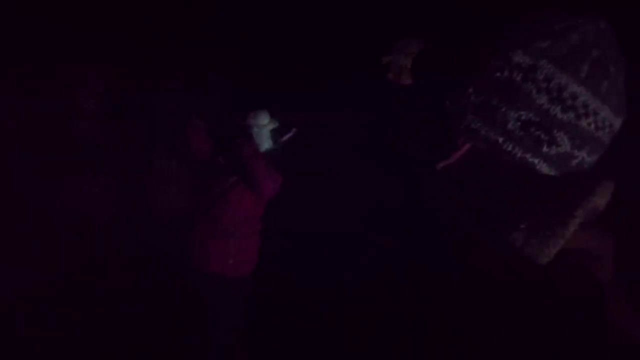 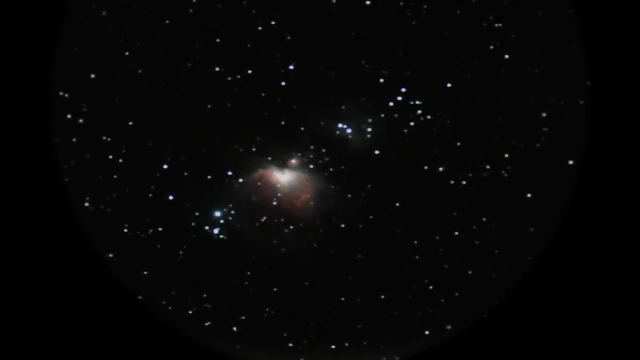 Anyway, the guys from the farm came out to have a look too, And their daughter. she could actually see it in colour. So I guess what it looks like also depends on how good your eyes are. It is pretty cool. It is cool. 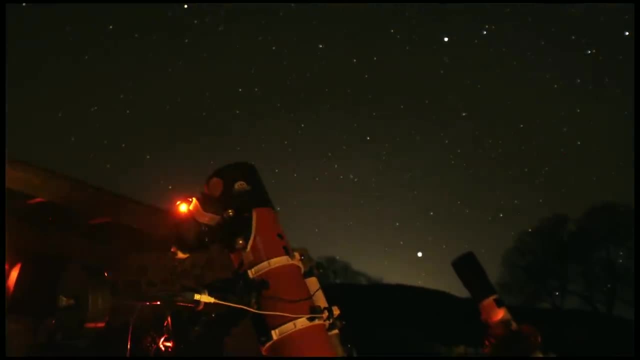 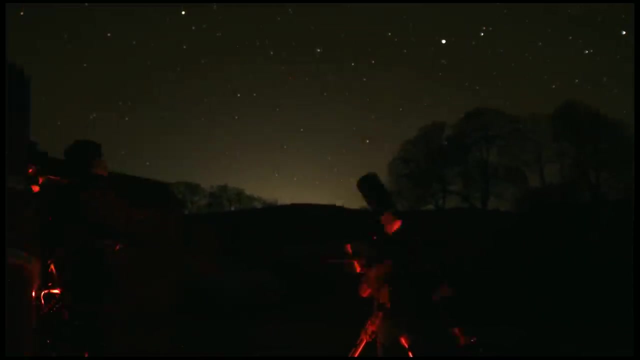 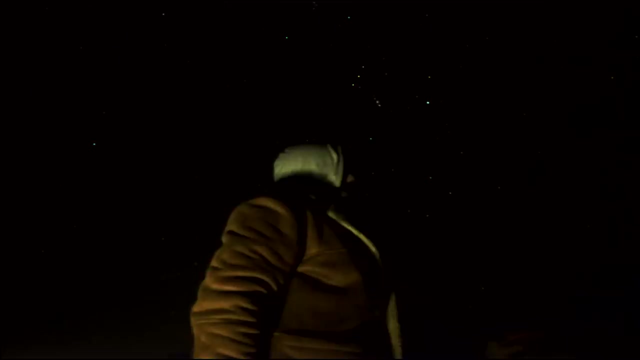 So the binos could pick up Orion's 12 light-year-wide ball of glowing gas. But now I want to have a look at some dust Dust around one of the most famous open star clusters in the night sky: Seven sisters- It's supposed to be seven stars, but it's loads more. 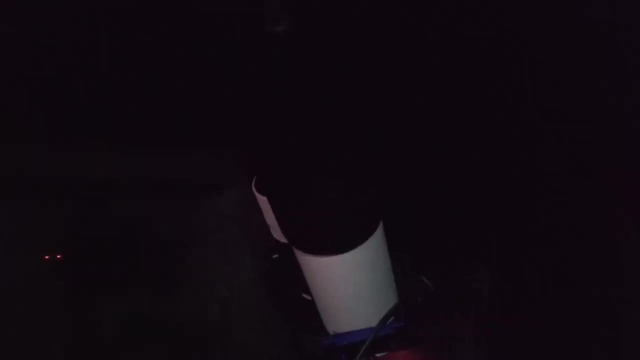 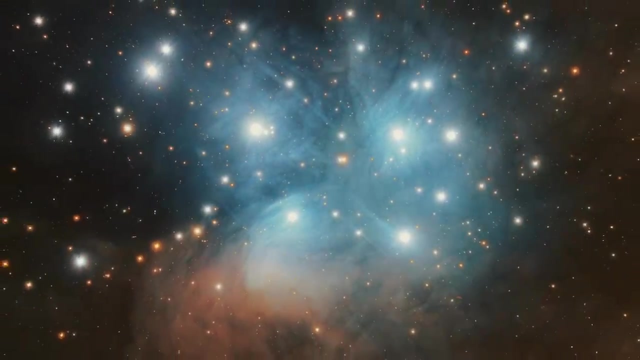 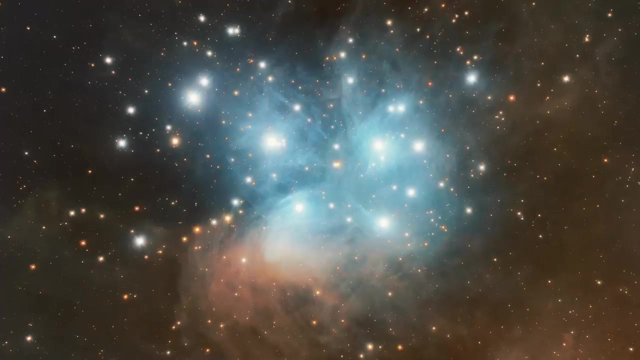 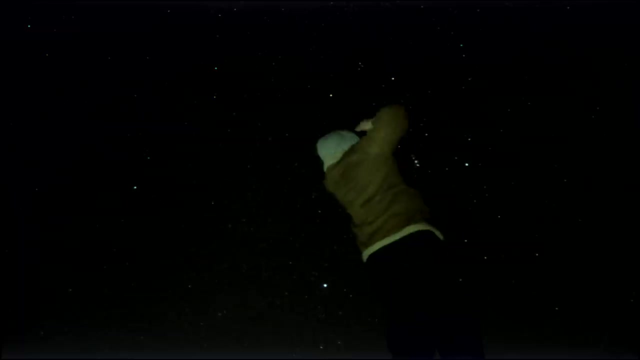 For an hour and a half my fancy telescope has been shooting the seven sisters And it is just gorgeous, Lovely, lovely dust lanes which are reflecting the light from those bright blue stars. It's gorgeous, All right, by any time. I mean pow. 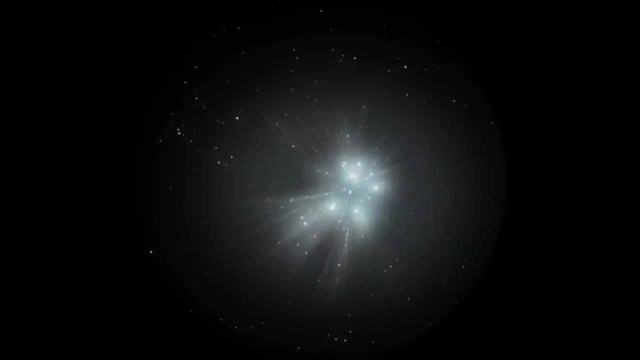 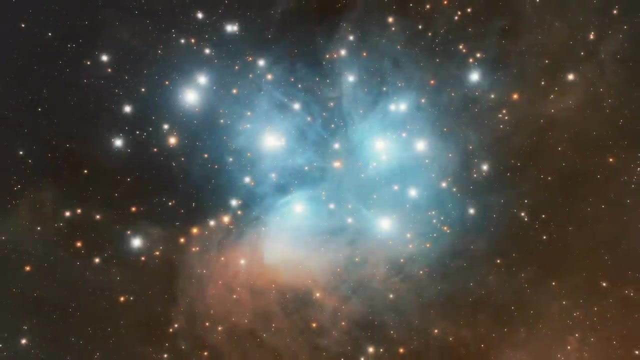 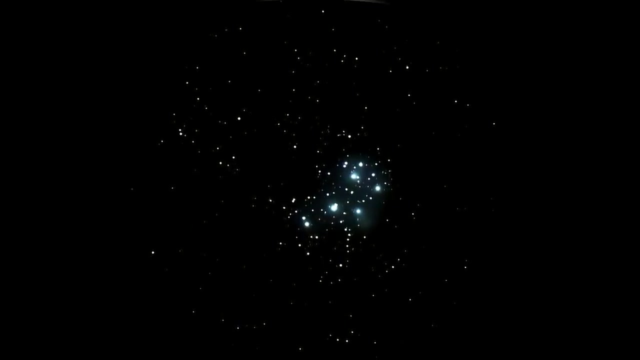 God, it's like. it's like looking at headlights, that's so. those seven sisters are so bright. Tell you what it looks. nothing, nothing like the photograph I've taken or what BinoCam is showing you. It's a super bright ball, an amalgamation of stars that are just kind of floating in space. 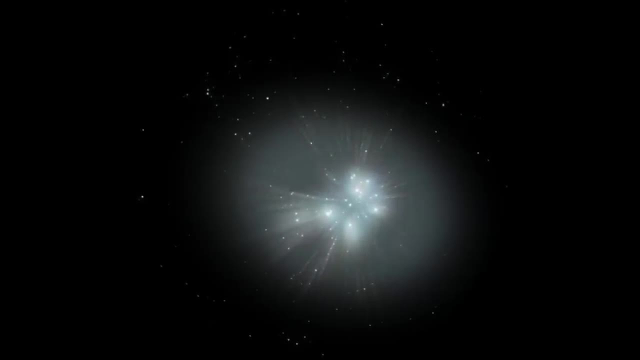 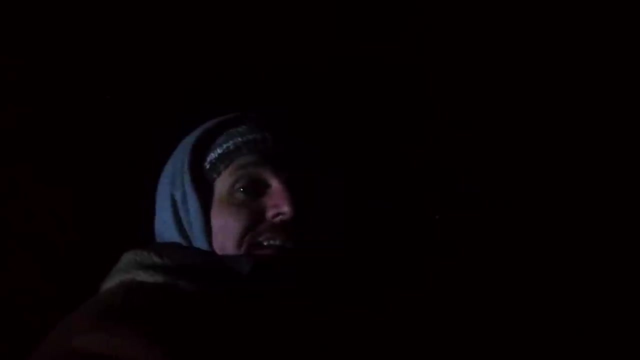 You don't get any of that from the photograph. But what about the dust? I'm not sure there's a sort of fuzziness. I can't. I can't honestly say I can see whisper dust like I see in the photographs. I spent another half an hour just cruising along the Milky Way. 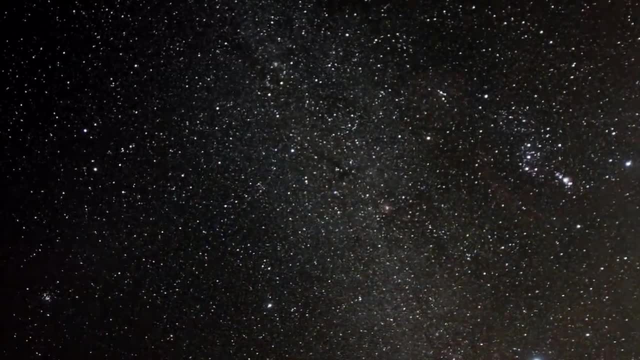 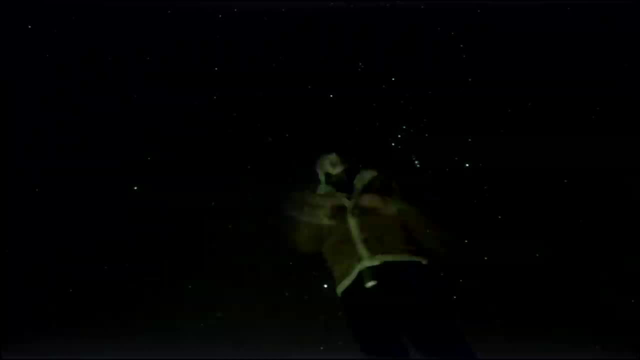 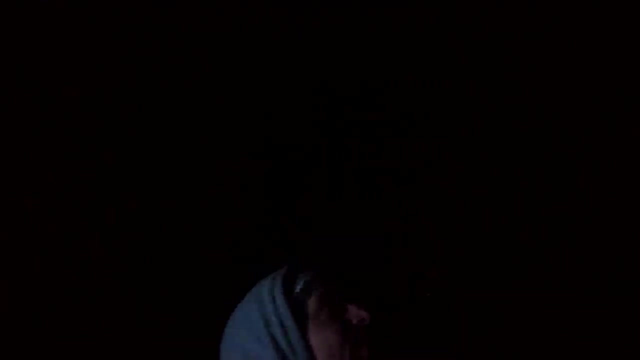 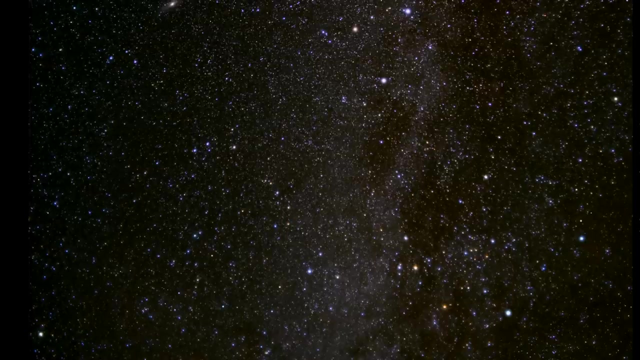 The Milky Way looks amazing. Then I decided to check out our nearest, biggest galactic neighbour- I think I can see it even without the binoculars. It's big. It's big. It's five times wider than the moon. To find Andromeda, what I did was follow the line of the Milky Way until I reached a W-shaped constellation called Cassiopeia. 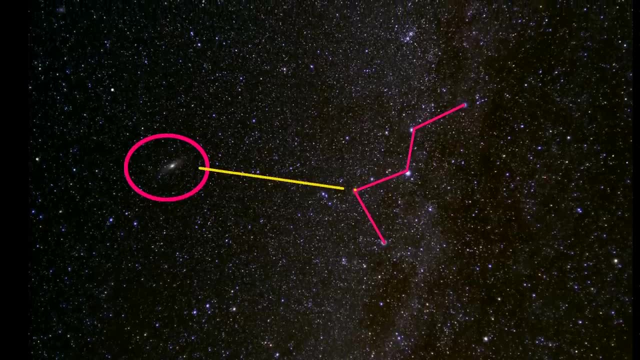 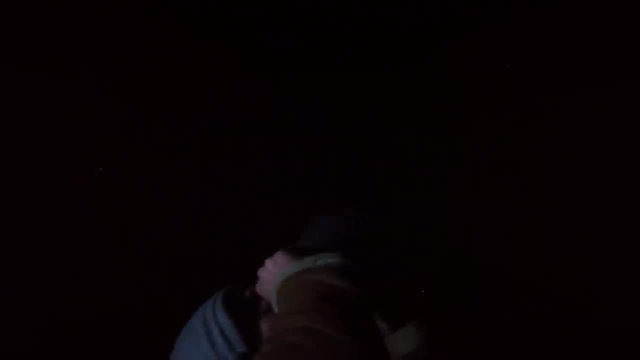 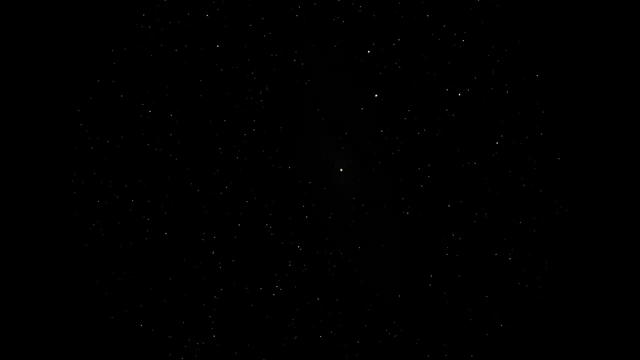 Now the bottom triangle sort of points to Andromeda. Wow, It's amazing And it's big. It's bloody, bloody, bloody, bloody big. At first I could just see stars With a faint smudge behind them. 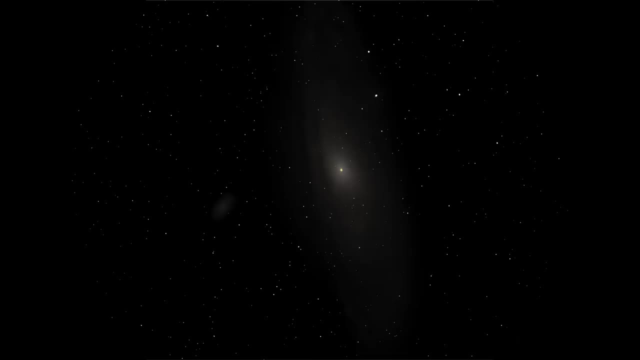 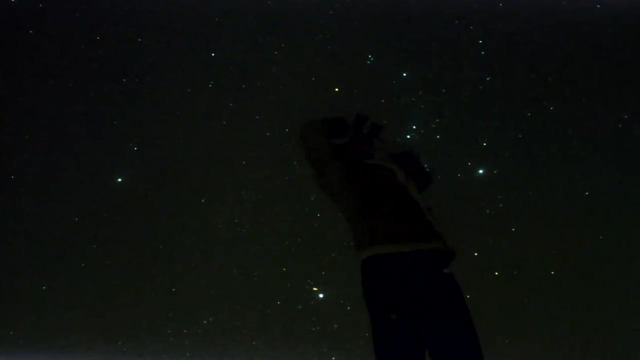 Then the smudge resolved into an ellipse And my knees began to tremble like I was on the edge of a cliff. How could something so big be floating above me? And it's just sitting there watching us? My heart is skipping a beat because that faint splurge is like 30 million light-years away. 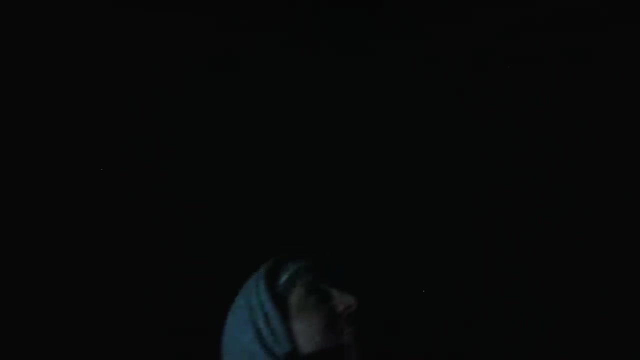 Andromeda. Andromeda is just mad, Mad, mad. I mean I can't explain it. It doesn't look, It's not like you see loads of stuff, But it's the thing that has most got me, for sure. 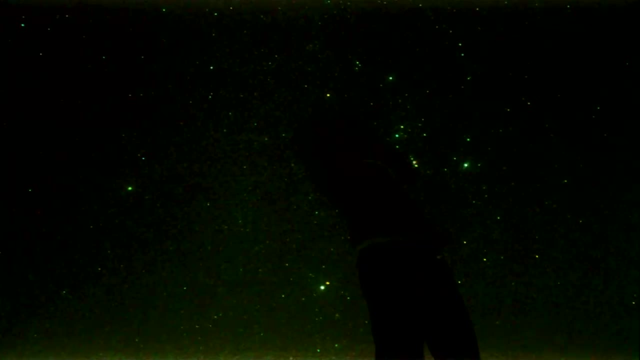 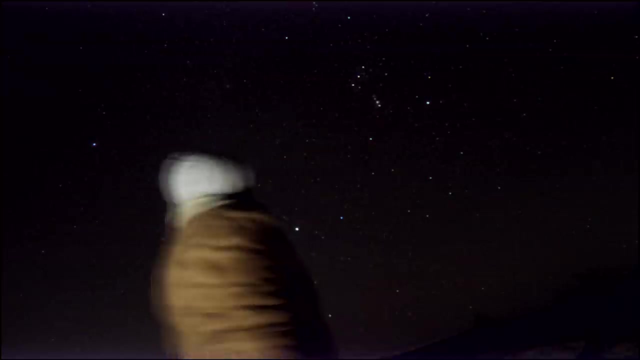 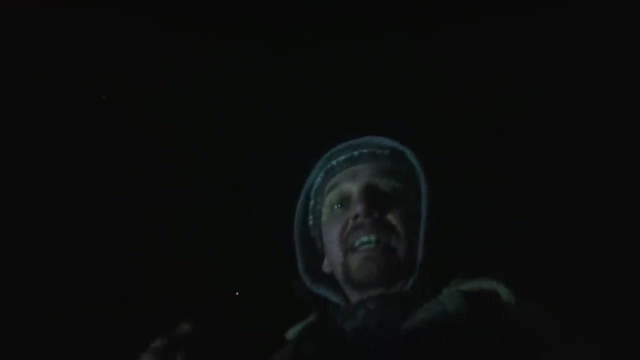 So, after two hours of looking through binoculars at the night sky and seeing stuff like this- the Rosette Nebula- what do we think? What's the verdict? Is it going to float your boat? I don't know. You ain't going to see. 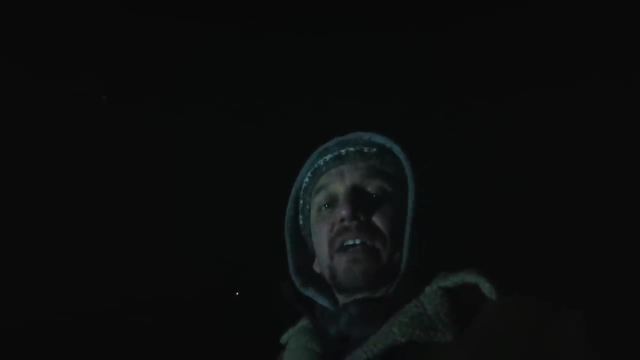 Like it's not going to look like it does in the pictures, But there's something about it being real And really being here and really appreciating it. That's cool, I would say. being outside somewhere really dark is magic.